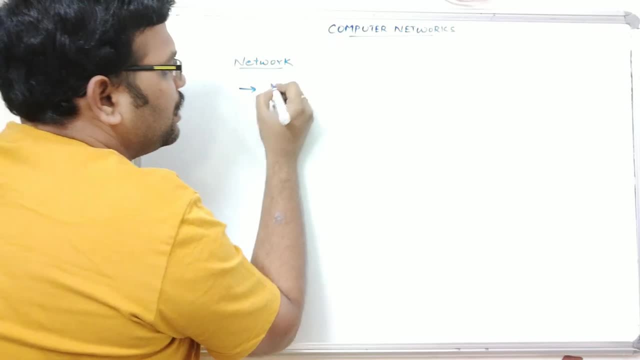 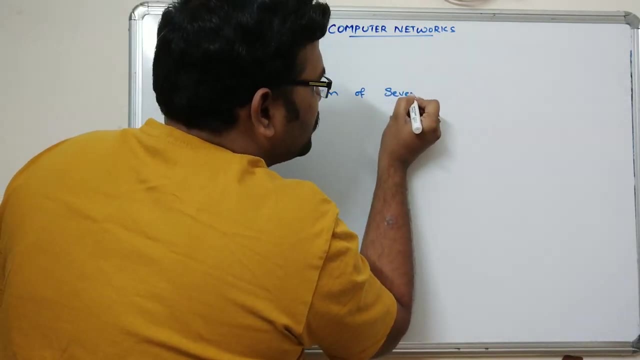 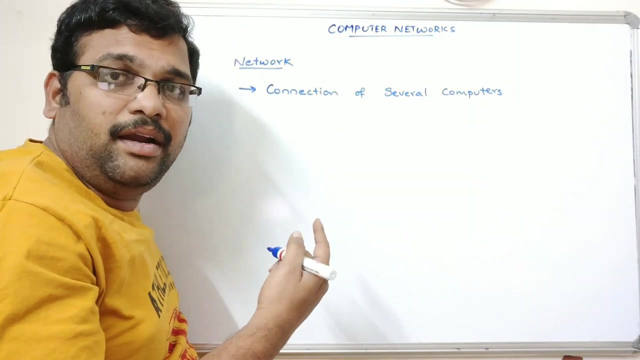 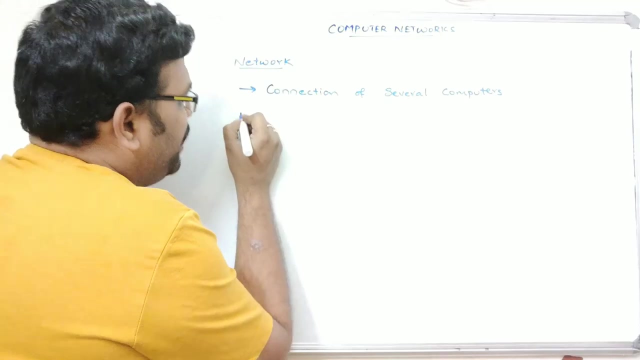 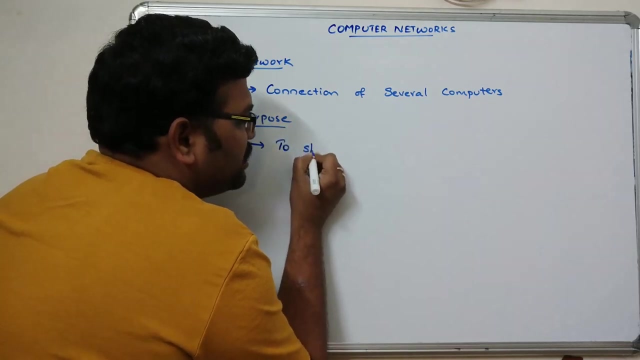 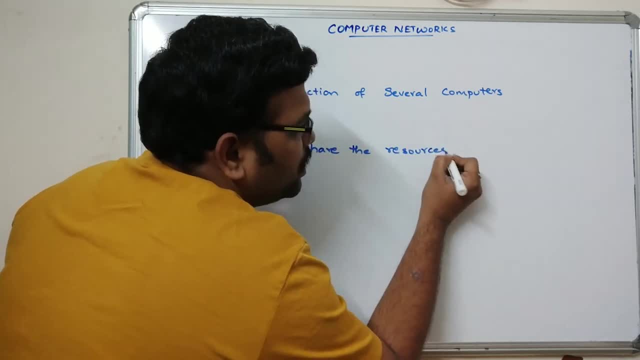 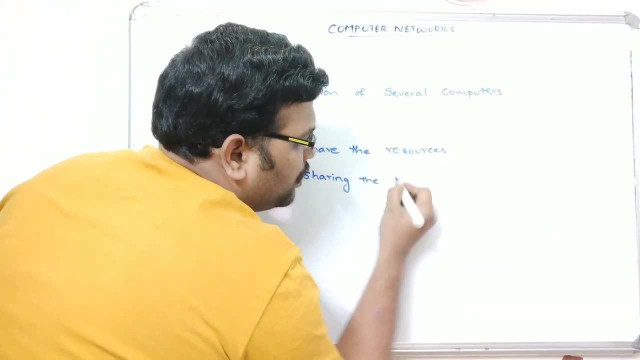 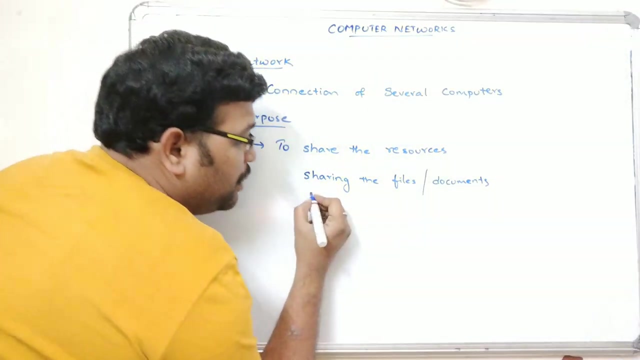 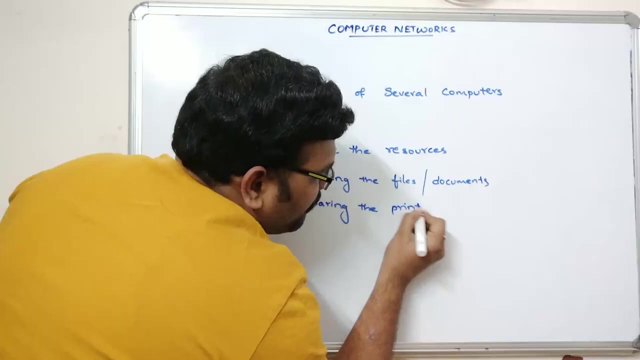 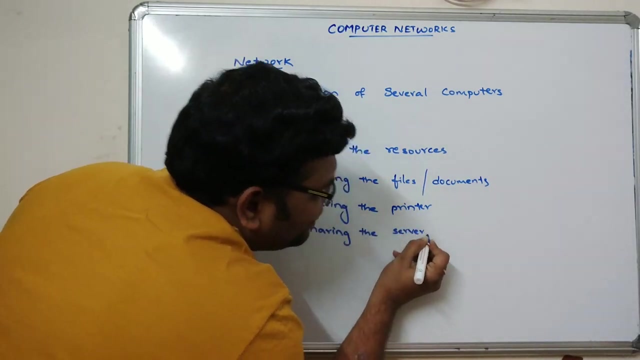 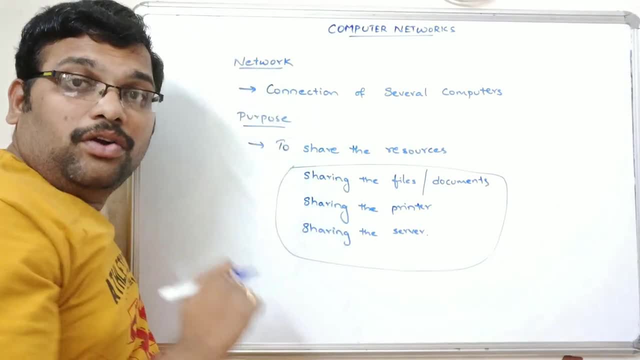 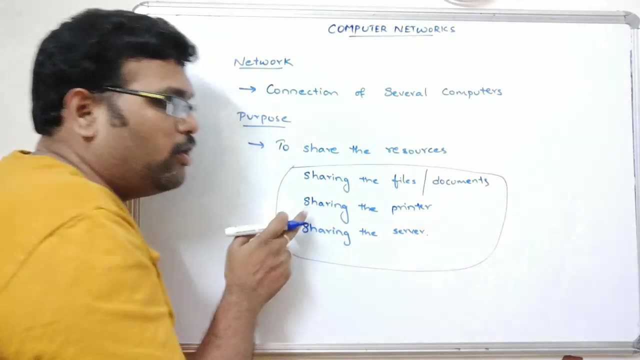 We connect several computers, which is called as a network. in order to connect these computers Will require some medium past, in order to share the files, or in order to share the printer, or in order to share the server. We are supposed to this computers with the help of some gast CPR network. 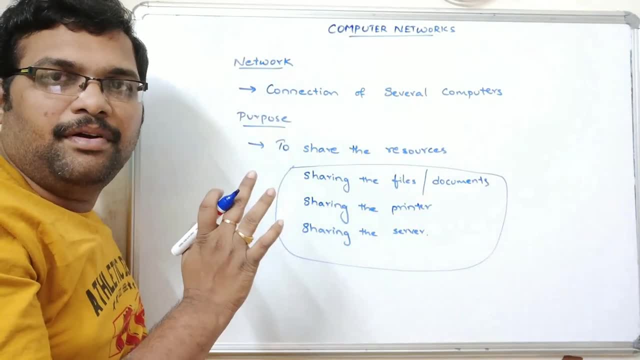 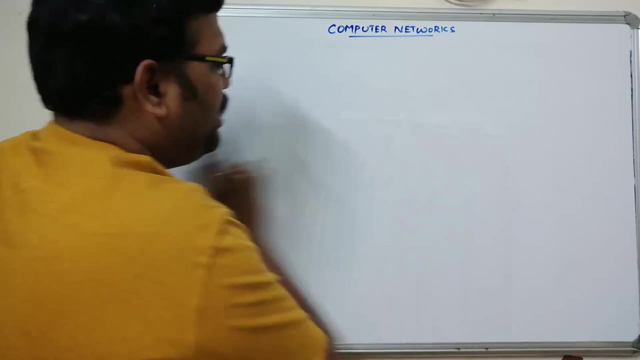 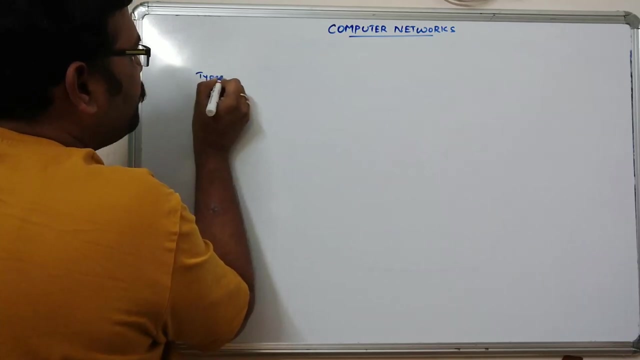 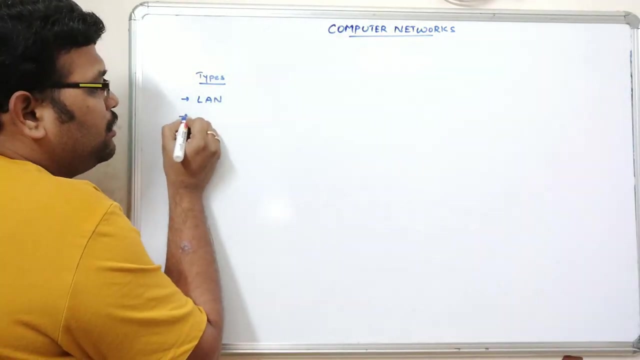 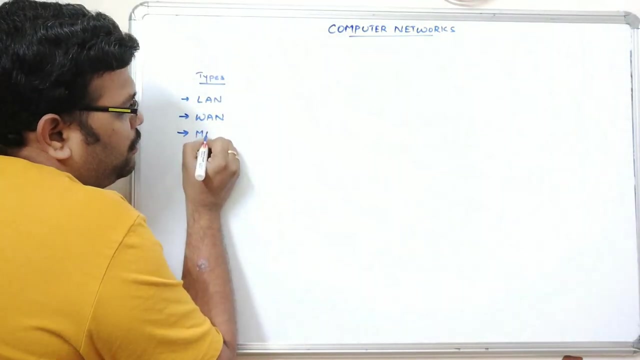 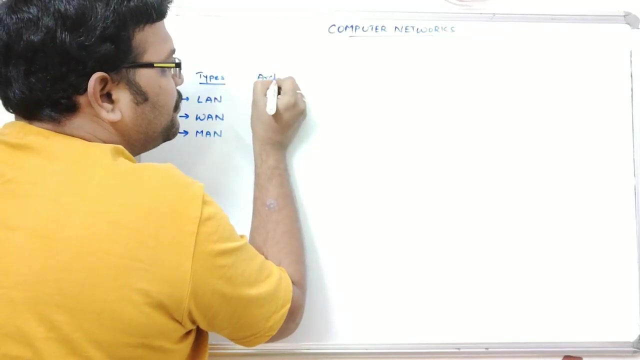 with the help of some transmission medium. right now there are different types of networks available. types of networks. so one is LAN, which is a local area network, then it's a wide area network, man metropolitan area network and, based upon the architecture, there are several, several types of networks. 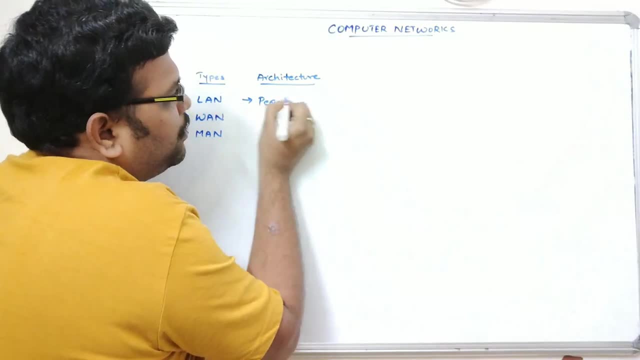 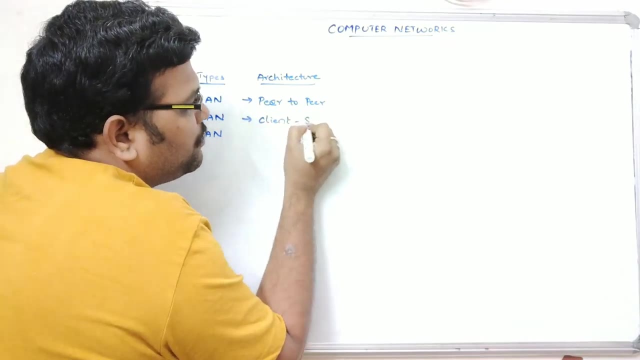 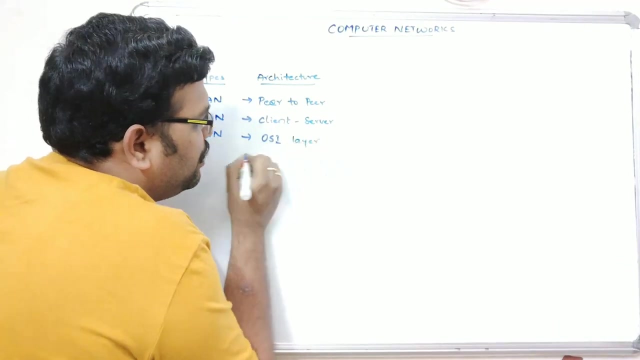 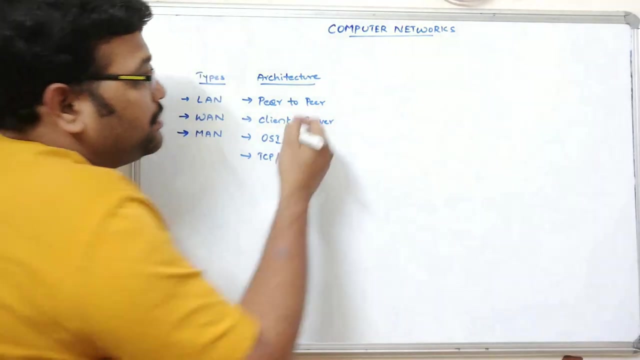 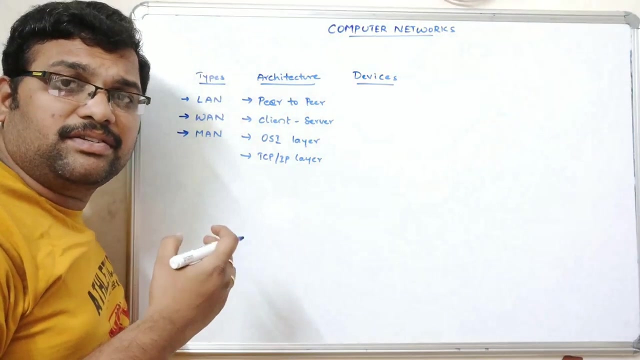 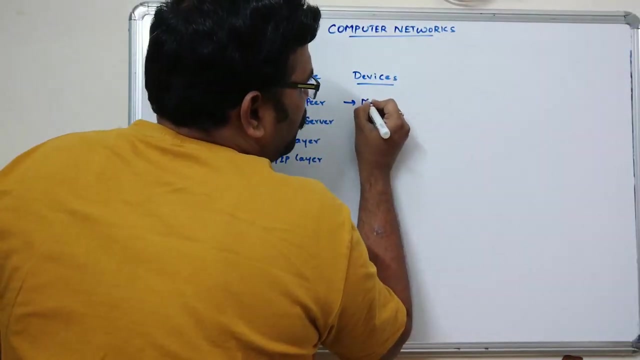 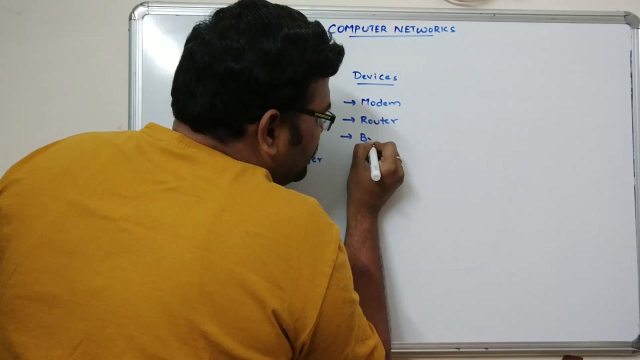 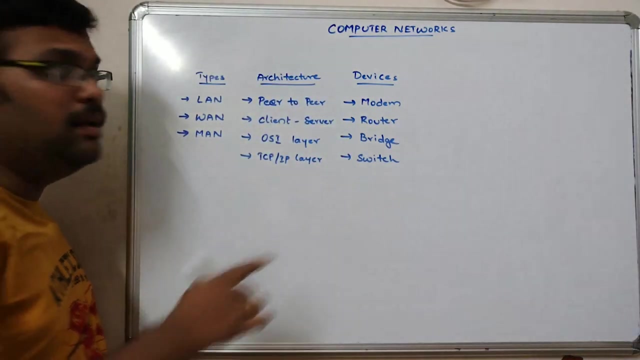 one is peer to peer network and client server network. Apart from these we will also learn OSI layered architecture and TCP IP layered architecture. All these things we will learn in the further sessions. Next, devices: So we will use a number of devices in this computer networks while going with the further sessions. Those are modem, router, bridge switch, etc. All these things we will learn in the further sessions. 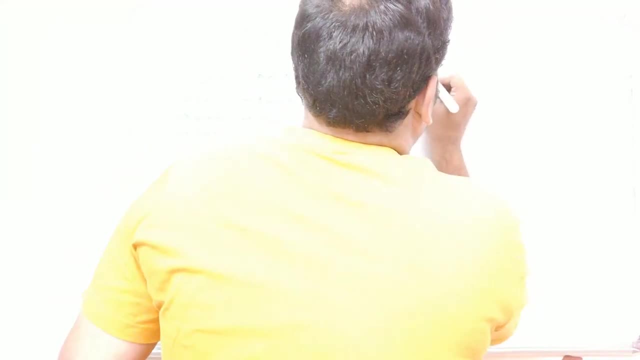 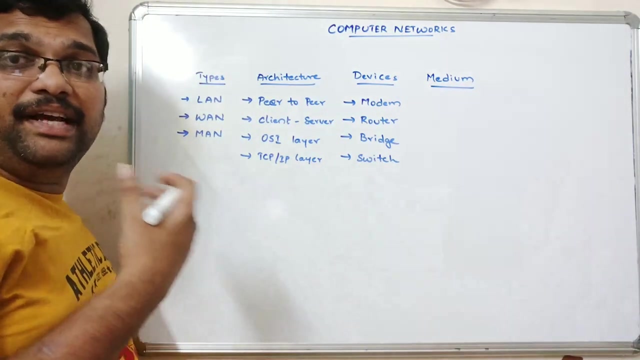 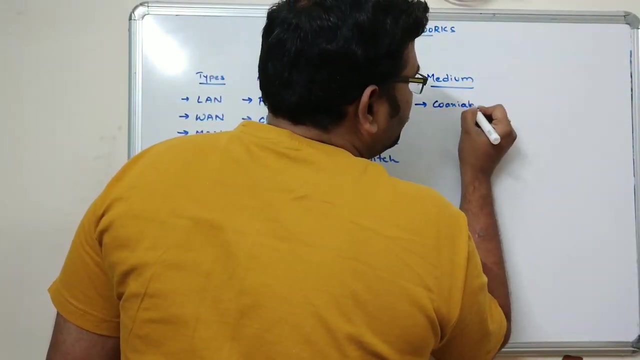 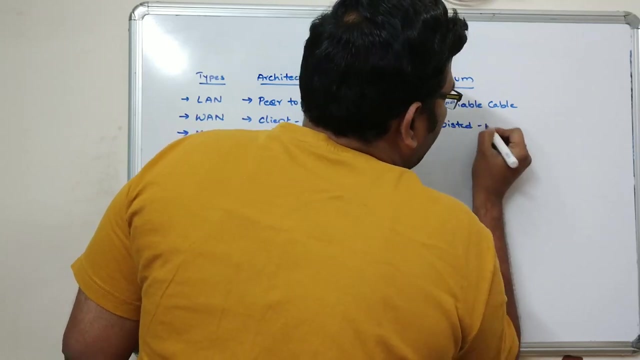 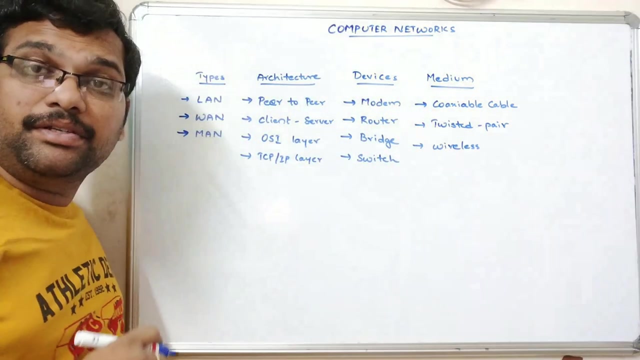 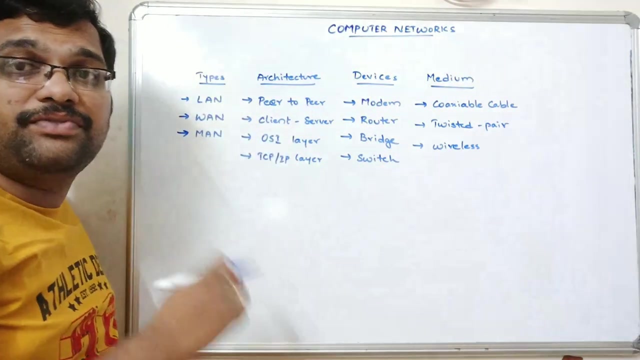 Next, based upon the medium, that means how we can share the files from one computer to another computer. Here we will use coaxial cable, twisted pair cable or wireless cable, Wireless networks. So all these things, with the help of all these things, we can connect several computers and we can share the resources from the one computer to another computer. 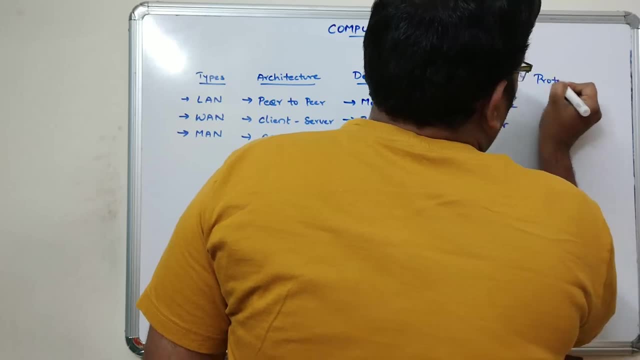 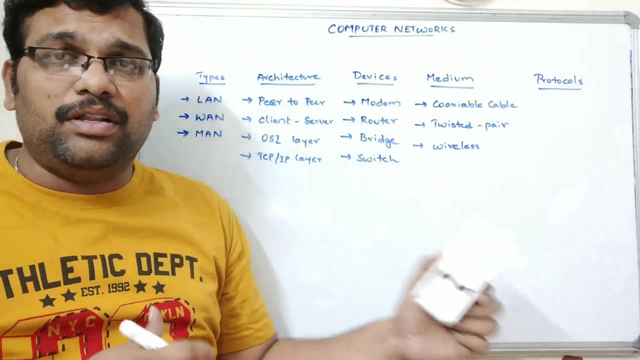 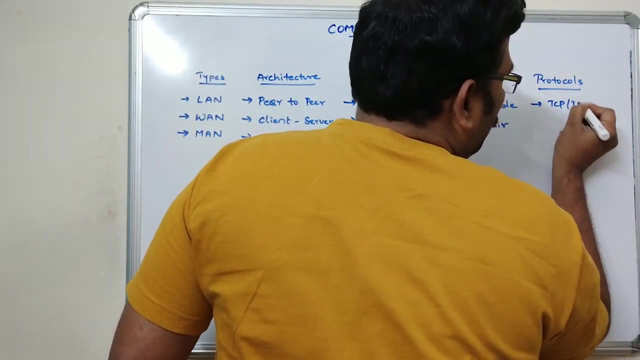 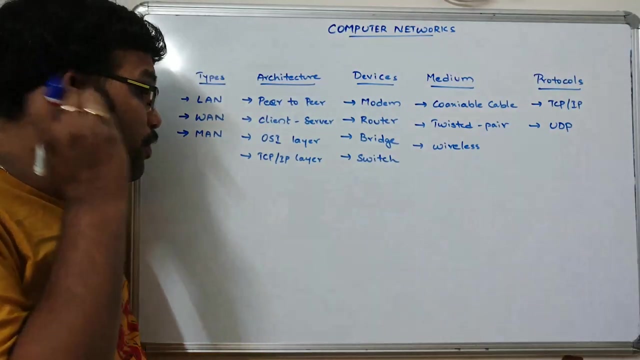 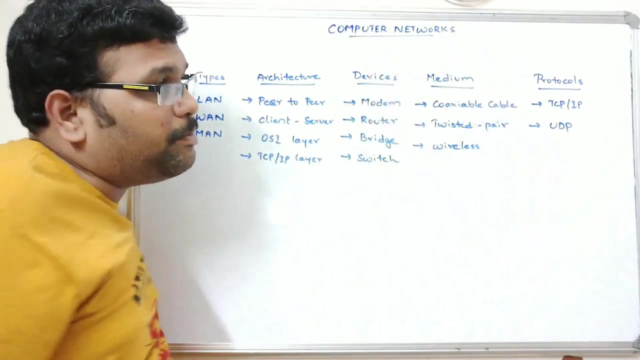 Next protocols. So in order to share some files from one system to another system, we have to follow some protocols. So here mainly we will follow the TCP, IP protocol As well as UDP protocol, So connectionless protocols and connection oriented protocols. So before transmitting or before sending the files from one computer to another computer, we are supposed to use any one among these two protocols: TCP, IP protocol or UDP protocol. 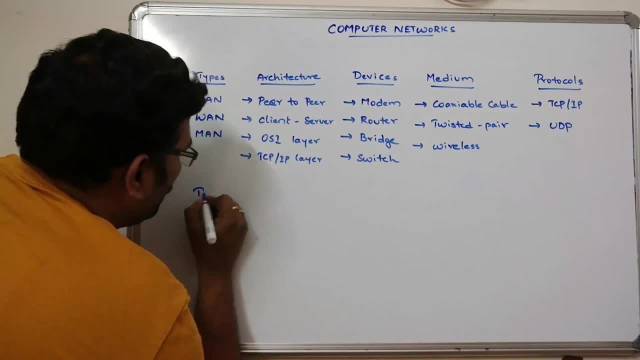 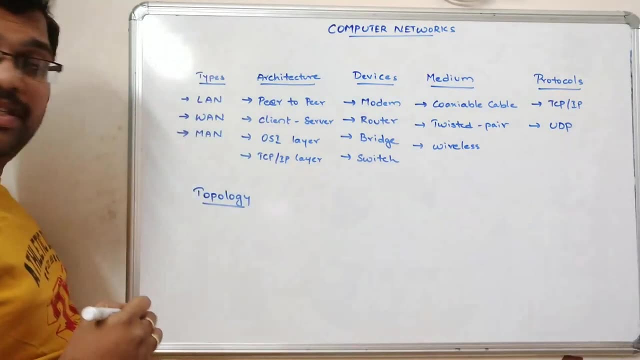 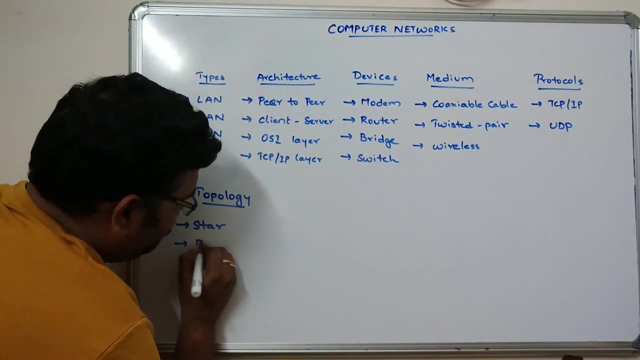 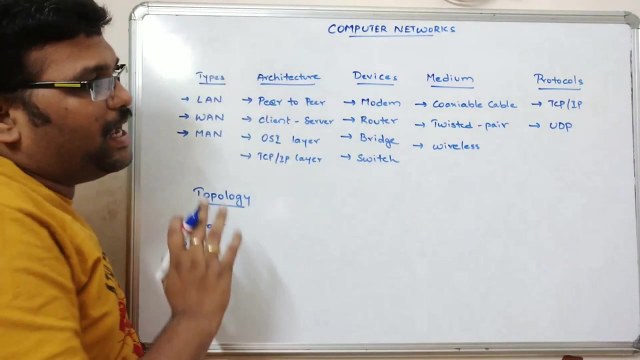 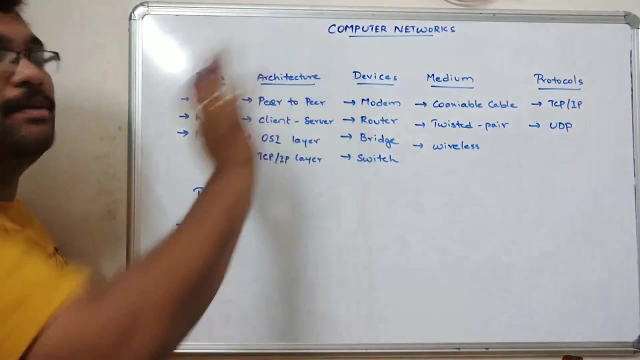 Then topology follows a different topologies. so there are star topology, bus topology, ring topology. so don't worry about these things. so this is just an overview of our further sessions. so we will suppose to learn all these things in this computer networks right topology. there are three topologies: star, bus.